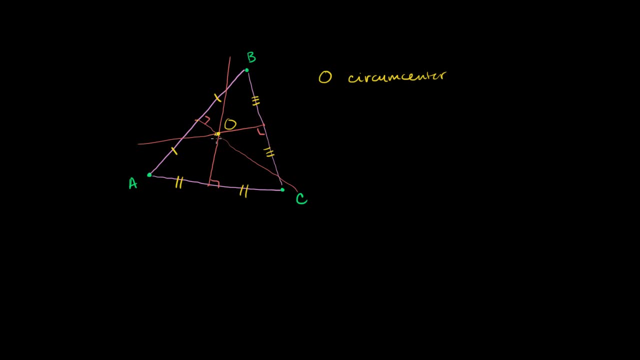 That unique triangle has a unique circumcenter which is equidistant to the three points of the triangle, I should say the three vertices of the triangle. And that distance between the circumcenter and the three points, the three vertices, I should say. 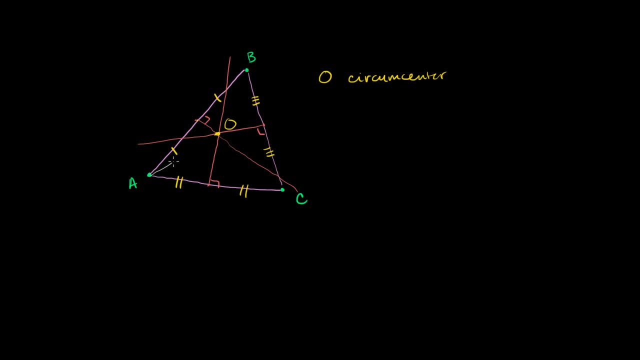 So let me draw that in a different color. So this distance, OA, the length of OA, the length of OC and the length of OB, So OA is equal to OC, is equal to OB, which is the circumradius, And we've learned when we first talked about circles. 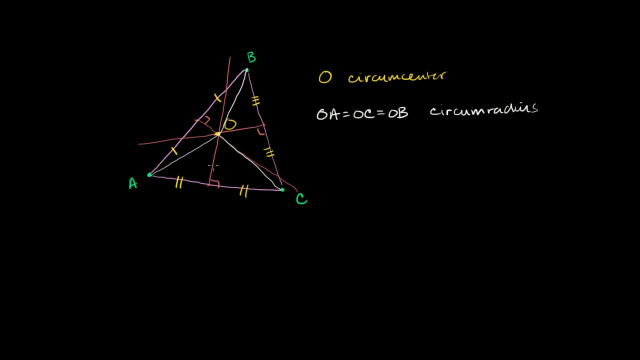 if you give me a point And if we find, If we find the locus of all points that are equidistant from that point, then that is a circle, And when I say locus I mean the set of all points. If you give me any point right over here. 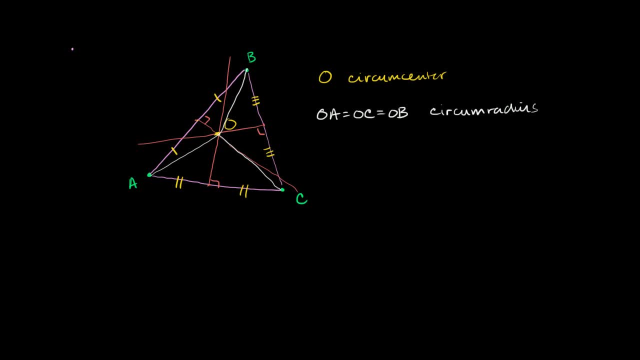 so that's an arbitrary point. and you also specify a radius and you say: what is the set of all the points on this two-dimensional plane that are equidistant, that are that radius away from the center? it uniquely defines a circle. 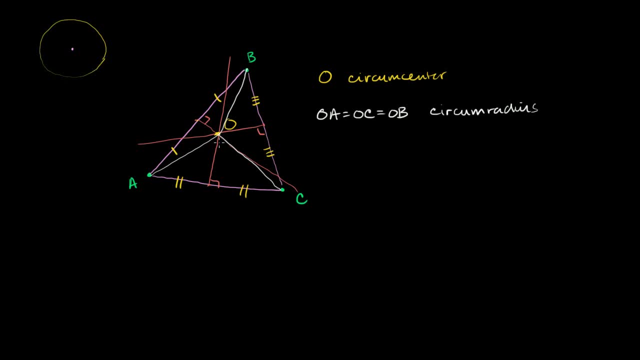 That's how we defined a circle right over here. And similarly, if you say, look, if you start with the center at O and you say all of the points that are the circumradius away from O, it will uniquely identify a circle. 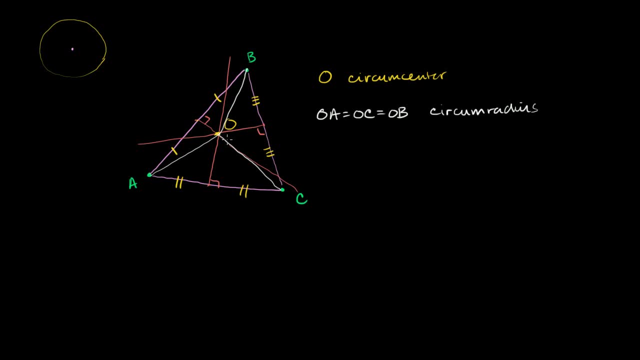 And that circle will contain the points A, B and C, Because those are the circumradius away from O, So they are included in that set. So the circle would look something like this. Draw my best to draw it just like that. 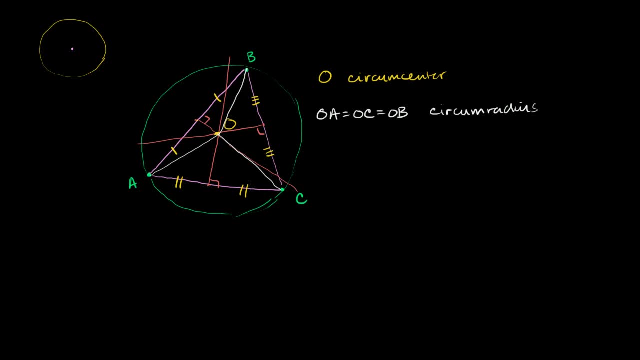 Now, everything we talked about just now, in the last few minutes, is all review. We know all of this, But I went over it just to kind of reinstate a pretty interesting idea: That if you give me three points, that defines a unique triangle. 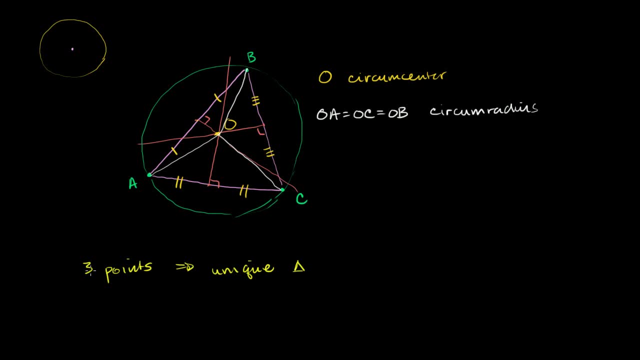 And if you have a unique triangle- and let me make it clear, this is three non-collinear points, So three points not on the same line, The same line. If you have three points that are not on the same line, that defines a unique triangle. 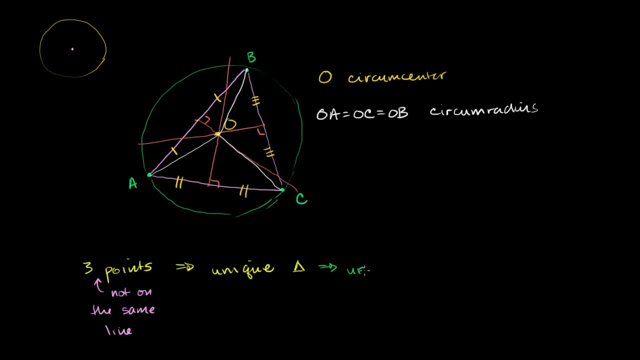 For any unique triangle you have a unique circumcenter, Unique circumcenter and circumradius. I'll rewrite it. I don't want to get lazy and confuse you Circumradius And if you give me any point in space, any unique point. 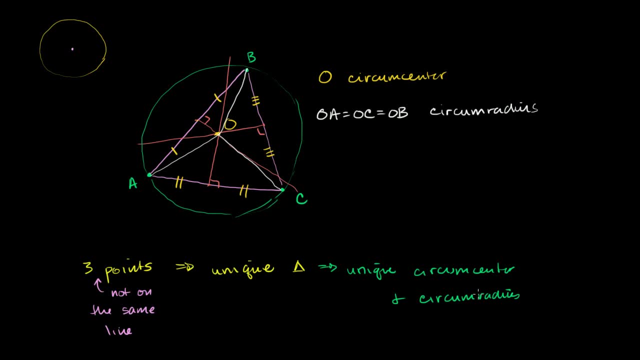 and a radius, the set of all points that are exactly that radius away from it. that defines a unique circle. So we went through all of this business of talking about the unique triangle and the unique circumcenter and the unique radius to really just show you that, if you give me any three points, 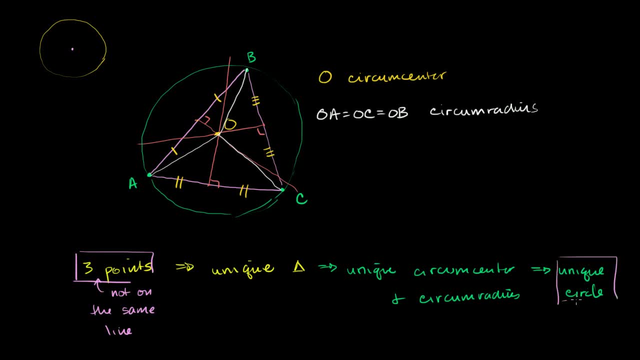 that eventually really just defines a unique circle. So just as you need three points to define a triangle, you also need three points to define a circle. Two points won't do it, And one way to think about it is, if you give me two points, 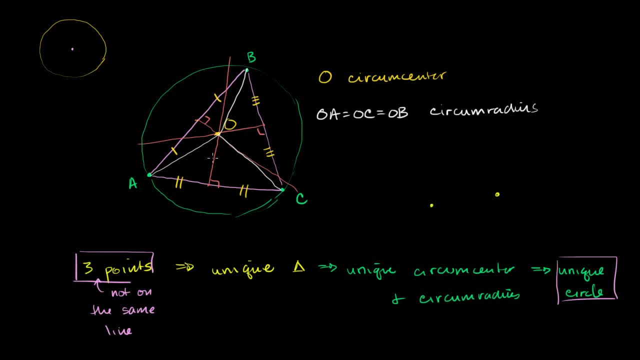 there's an infinite number of triangles that I construct with those two points, Because I can put the third point anywhere. I could construct this triangle, I could construct this triangle, I could construct this triangle, I can construct this triangle, And all of these triangles are going. 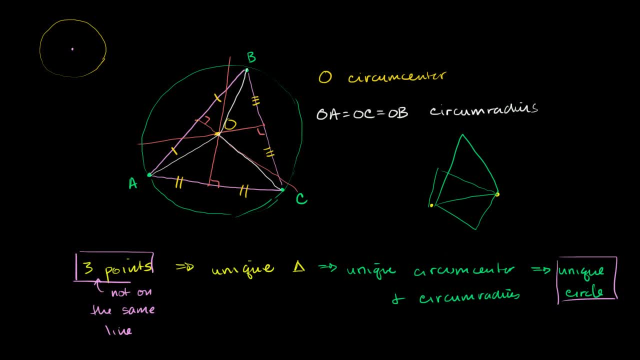 to have different circumcenters and different radiuses, And so they're going to have different circles that circumscribe about those triangles. So, for example, this would be one circle that could circumscribe that triangle. You could have this circle right over here. 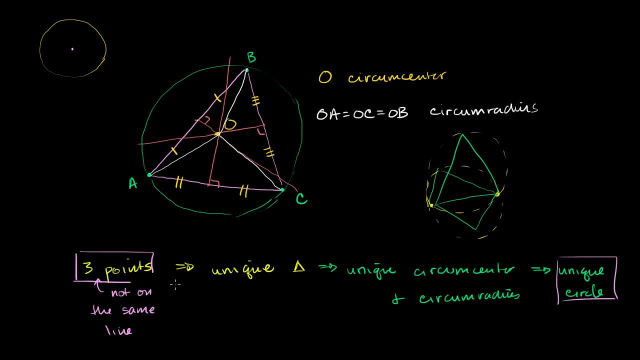 So you see very clearly that two points are not enough. You need three points. Three points lead to a triangle, You lead to a unique circle. So that by itself is kind of cool. Now another question is if I have just a circle. 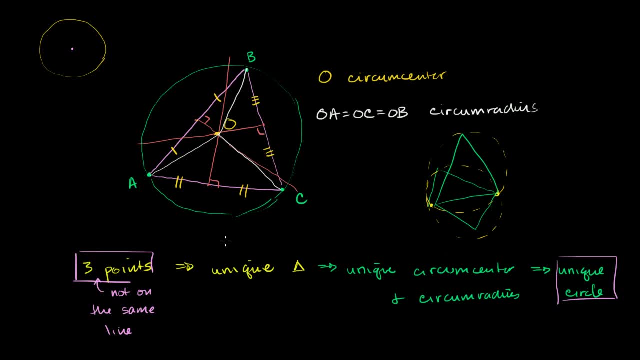 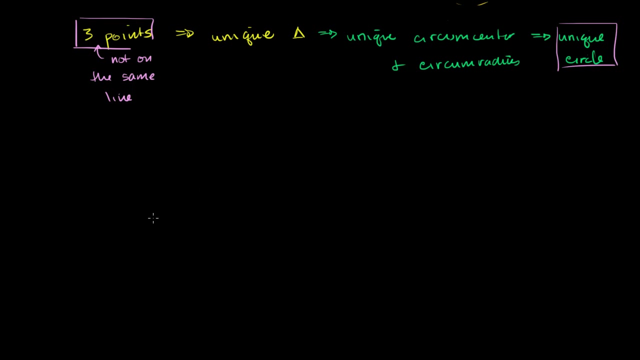 and if it's circumscribed about an arbitrary circle, is the center of that circle necessarily the circumcenter? So let's think about that a little bit, Because there are some, I guess, unnatural, or I wouldn't say unnatural- non-intuitive cases here. 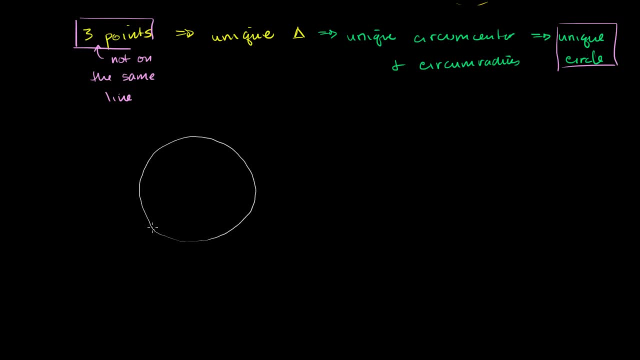 So if I draw a circle right over here, its center is right over there. And if I draw an arbitrary triangle where all of the vertices of that triangle are on this circle, is this center necessarily the circumcenter Of that triangle? So let me draw a crazy situation. 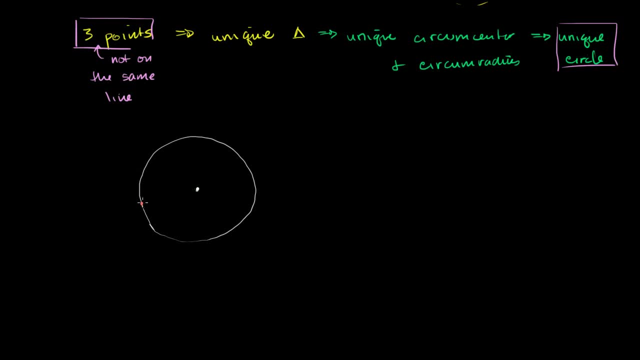 So let me draw one where this thing is clearly outside of the triangle. So we could have a triangle that looks like this And it's clearly all three vertices sit on the circle. So you might at first say, wait, there's no way this could be the circumcenter. 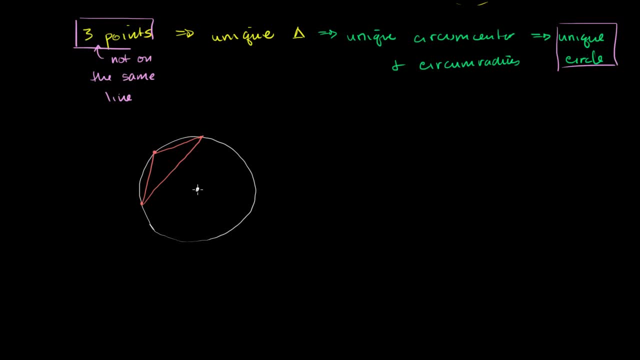 It's not even inside the triangle. But remember, this point right here is equidistant to every point on the circle. I should say every point on this circle is equidistant from this point. They are all the radius away And all three points of this triangle are on the circle. 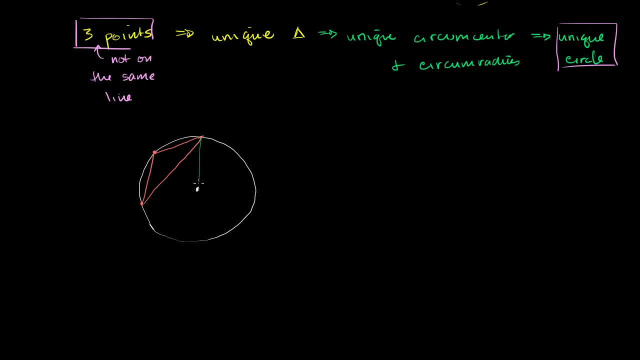 So they are all exactly a radius away from this point right over here. So this distance right over here is going to be a radius. This distance right over here is going to be a radius, And this distance right over here is going to be a radius. 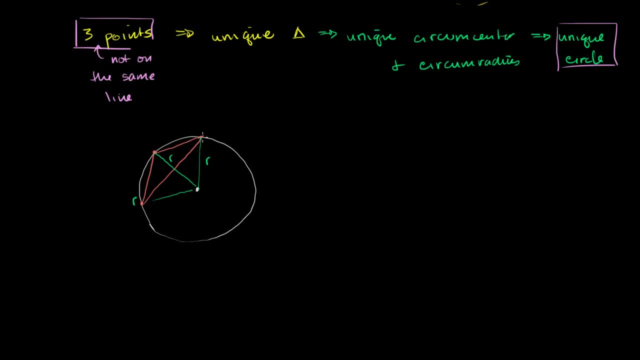 Now this point is clearly equidistant from that point and that point We know that It's exactly r away from both of those vertices of the triangle. So if it's equidistant- and we proved this in a previous video- 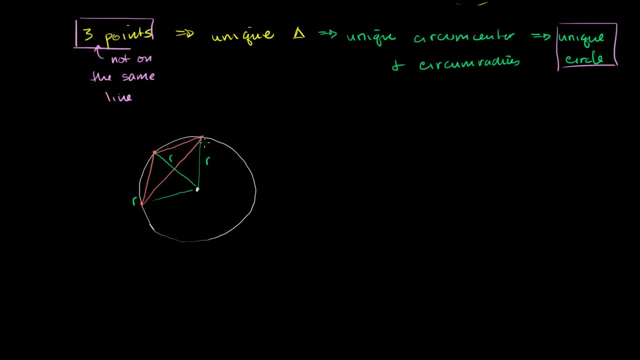 if it's equidistant. If it's equidistant from both of those points, it must be on the perpendicular bisector of the segment that joins those two points. So this must be on the perpendicular bisector. So it's perpendicular and it bisects that segment. 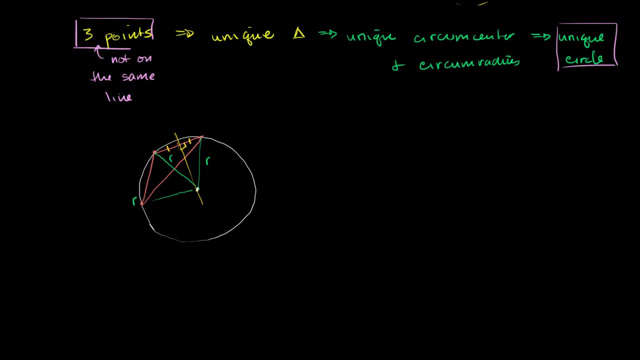 right over there, But we can make the same argument for this segment right over here, Because this point is r from the center. Oh, I'm tired of just saying this point. Point O is equidistant from. let me label these. 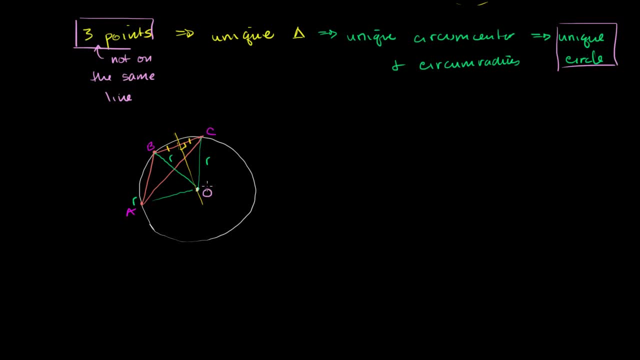 So let's call this a, b, c. So we already said, point O is equidistant from c and b, So it must be on the perpendicular bisector of b, c And it's also equidistant from a and b. 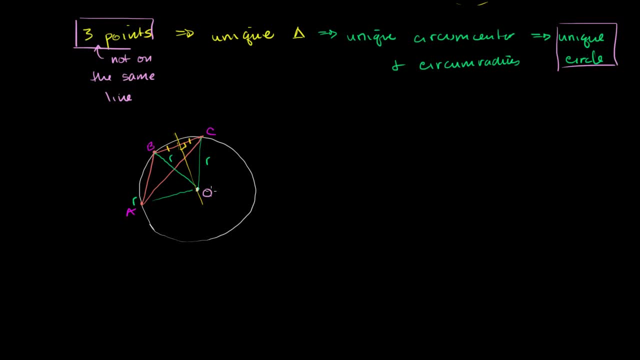 It's r away from both, because a and b both sit on the circle. They're both a radius away from the center, So it also must sit on the perpendicular bisector of a- b, So it also must sit on the perpendicular.